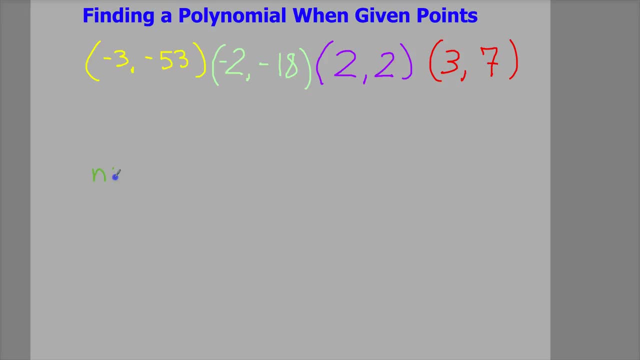 n. well, not in that color. that is not helpful at all. Let's try this n plus 1 point principle, And it's the idea that if you have two points, no matter what, as long as they're in the same plane. 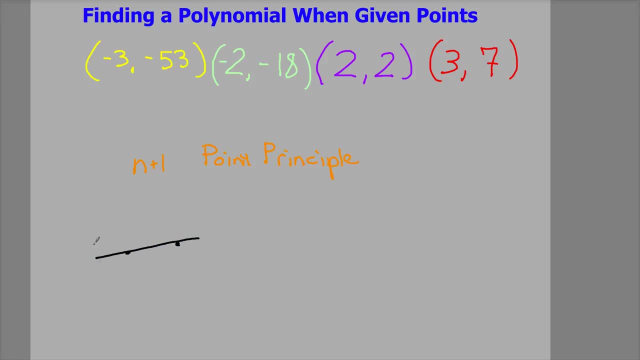 as long as they're in the same existence, not the same plane. they'll make their own plane, But if you have two points it'll be a line. This is all assuming, by the way, that these points meet the requirement for the vertical line test that passes a vertical line test. 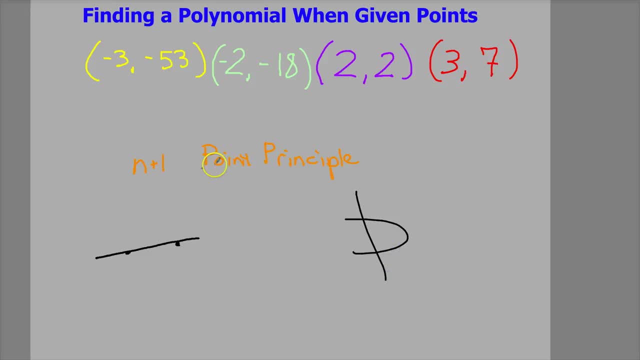 which is to say it doesn't curve back in over itself. This would not. the n plus 1 point principle won't work then. But if you have two lines or two dots or points, as they were, you'll have an x, so the x's of 1.. 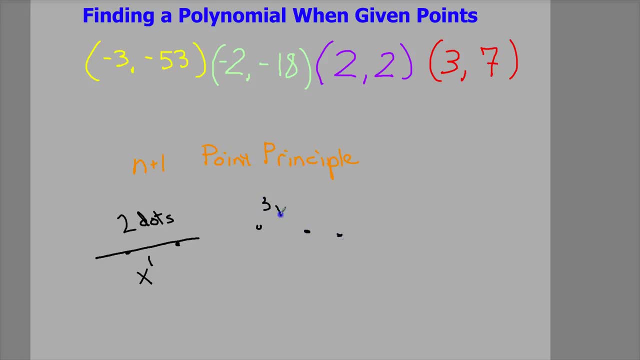 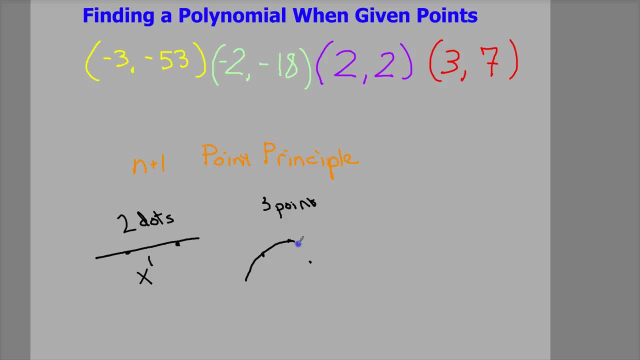 unless they're on the same line. I'm going to have to have some bit of quadratic structure. So if you have three points, x squared. If you have four, you know it's a bit of a x to the third power. 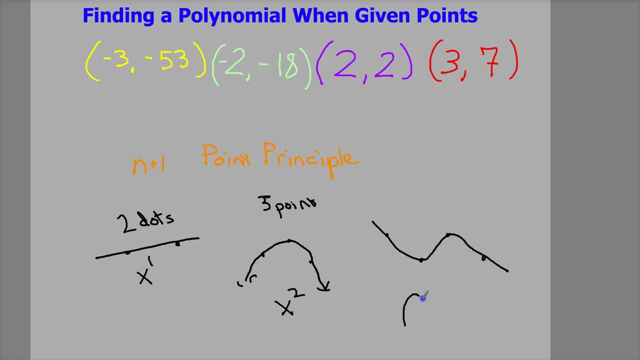 even though I drew them really close together and I wanted to have it look a little bit more like this. But anyway, if you have it you're dealing with the idea of four points will give you sort of an x to the third. So the idea behind it is that if you have this number of points, the n would be the degree. by the way, 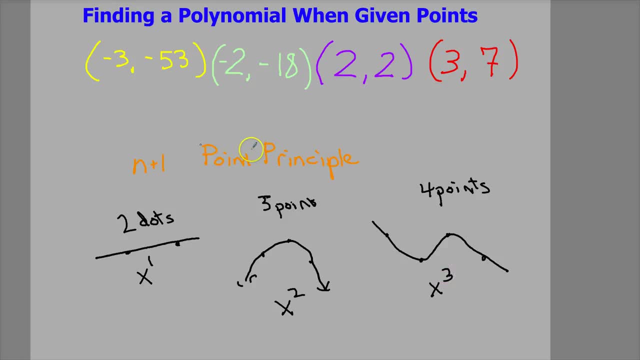 So, whatever the degree is plus, you'd have one more point. So if I have one, two, three, four points here, I can say that this graph is going to be x to the third power, That's going to be the highest degree on my leading term. 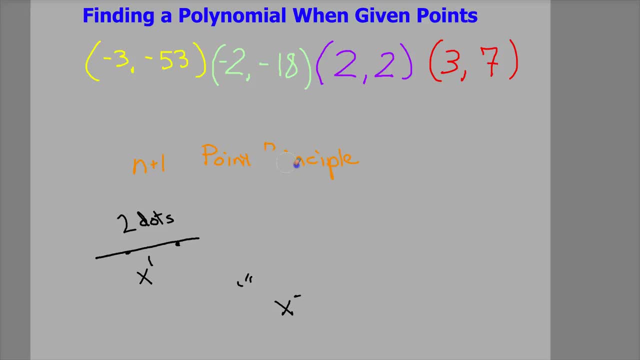 So let me erase all this out. Now, what do you do with that? Well, the idea behind it, now that we know that it's cubic, is that we need to write out the standard form of a cubic. So we'll do. y is equal to x to the third. 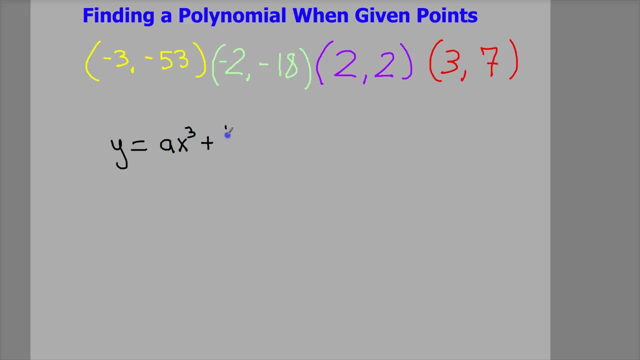 And we're going to put an a in front of it to cover for the coefficient plus b x squared, plus c x plus d. That's a generic form of equation. Where we go from this is I'm actually going to make what would be rows, essentially in a matrix, by plugging in these values to the equation. 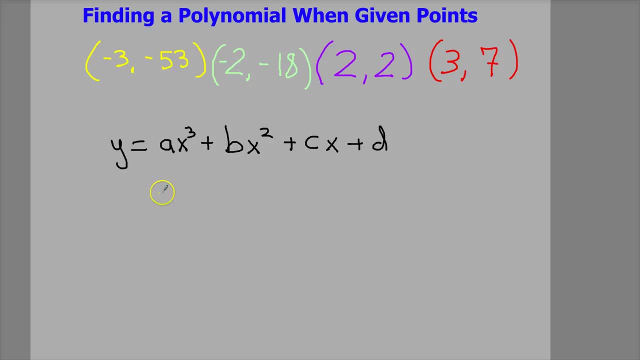 So for the yellow one, I'm going to end up doing I'm actually going to move the y equals to the other side, Just So it sets up the way it's supposed to set up when I turn it into a matrix. So this would be: equals y. 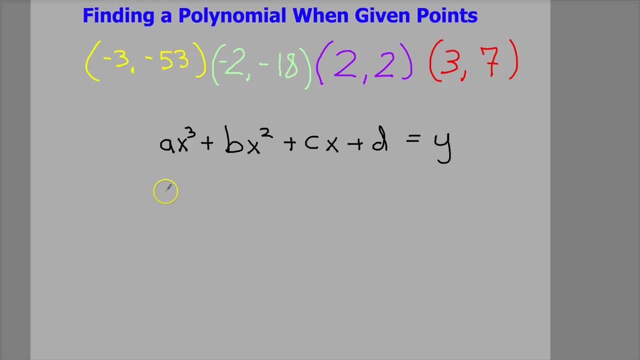 So for this one I'm going to do negative three in place of x. So a times negative three to the third plus b times negative three squared plus c times negative three plus one d is equal to my y value Of negative fifty three. 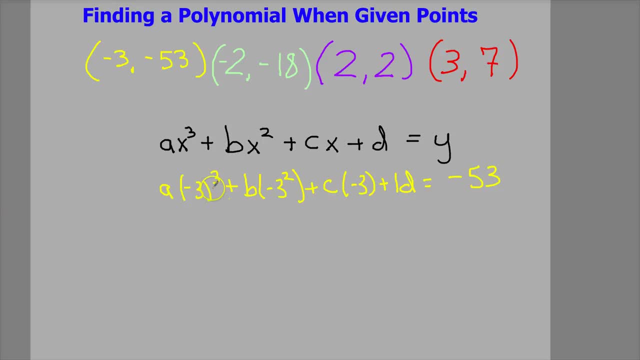 Now what that goes into, or what it becomes anyway, is I'll do negative three to the third power and get negative twenty seven a And then negative three, squared of course is nine. Make sure you put the negative three in parentheses. 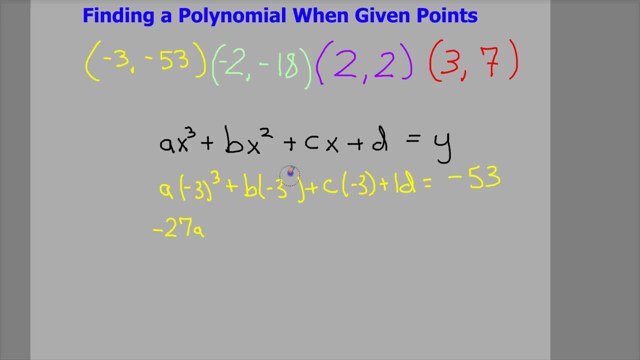 I don't know why I put the square inside, but it should be on the outside. Don't do what I did, Like this. You'll end up getting plus nine b and then negative three c. C plus one d is equal to negative fifty three. 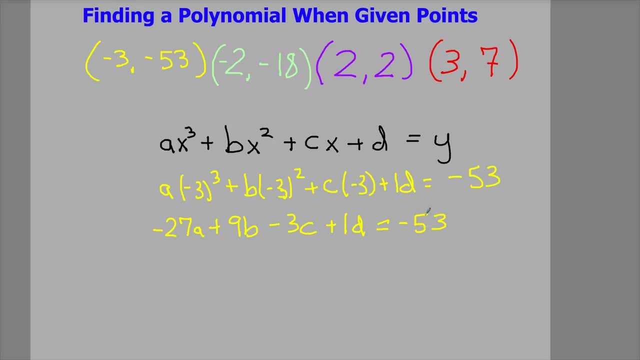 Now, from here, I'm actually going to go through and write out the other, The other three, and move this one up a little bit. So I'm going to pause the video. so you don't have to sit here and watch me do it, because it'll take a little bit, a little bit of time. 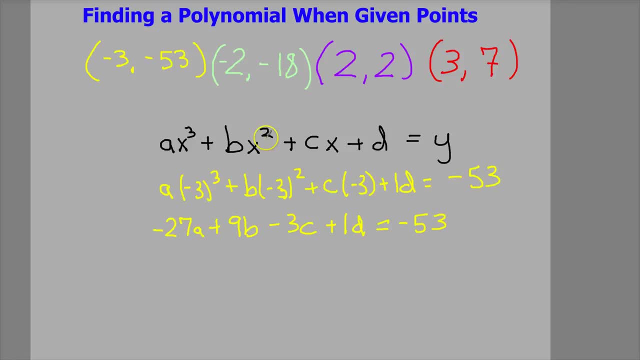 But essentially I'm going to take this negative two and plug it in for x and set it equal to negative eighteen, And then I'm going to do the same thing for the positive two, Plug it in for x and set it equal to two, and the three and plug it in. 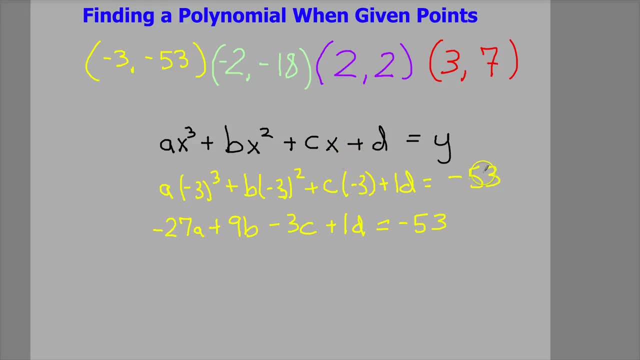 For x and then put the seven for the y. So in just a second I'll be back. You probably won't even notice any real time moving, and then I'll be back and explain where to go from here. All right, So now that I have all of these here and ready to go, I have them organized in a nice set fashion. 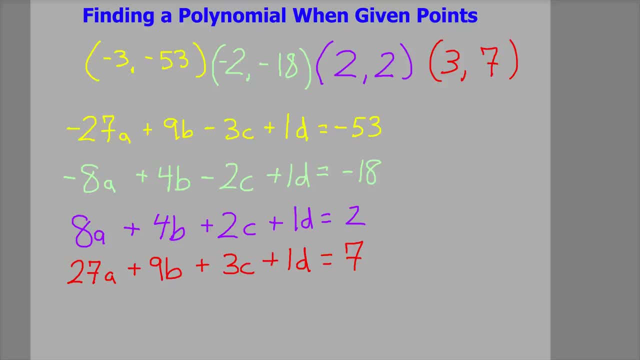 It'll look in standard form. So really, so far, what we've done is figured out that if you have however many number of points that you have, you subtract one and that will tell you the overall shape of your polynomial. So if you have five points, that means 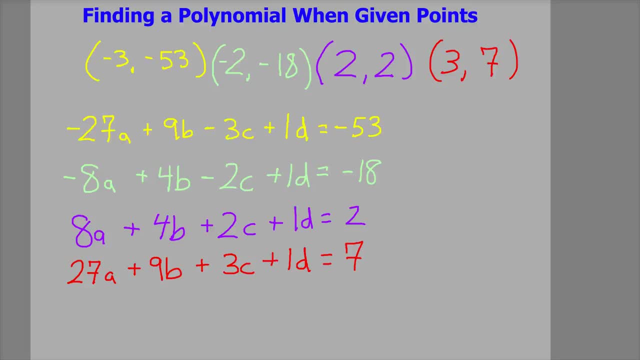 You can have four x to the fourth would be the most. then you need to write the standard form as it is of that. So y equals x to the fourth, plus, or so be a, x to the fourth plus b, x to the third plus c, x squared. 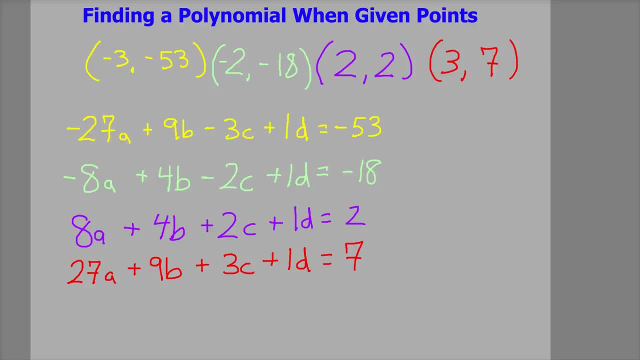 That whole thing. work those out, and then what you'll do is plug your x values in and set them, and then plug your y values in as well. Substitute, I should say. plug in is an evil word. now substitute your x values and your wise. 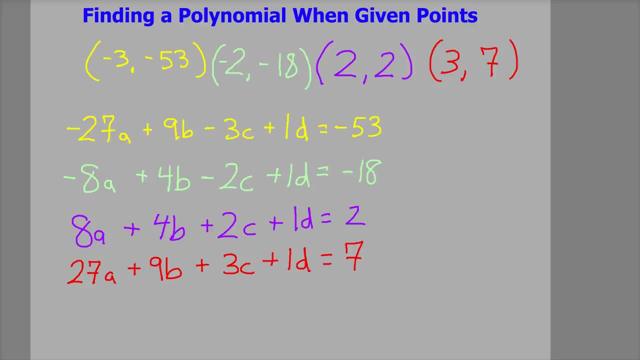 Make sure you put any negatives in parentheses. Give you that, and then you'll have this set up. What we're going to do is actually convert all of this into a nice matrix, So when I have these, it's going to look like negative. 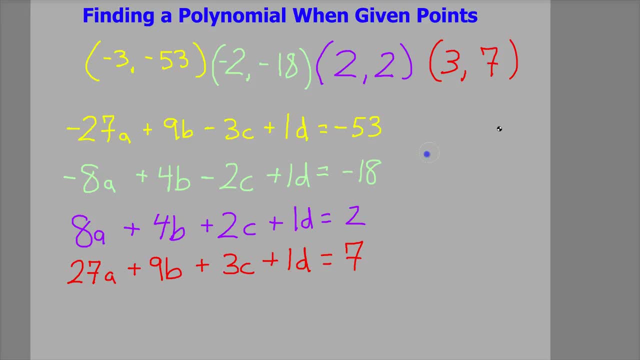 It's not the best color for this background, Just use this and be lazy. Negative: 27.. 9 negative 3, 1 negative 53.. That's our first row And then in the next one I'll do a negative 8, 4. negative 2, 1 negative 18, 8, 4, 2, 1 and 2. the big key here is to make sure that for your final value fits D or whatever letter happens to be, you put a 1 there, because if you don't, it will drop out. fit the system. the system won't work. you can't do what's called reduced row, echelon form. you won't evaluate it properly. 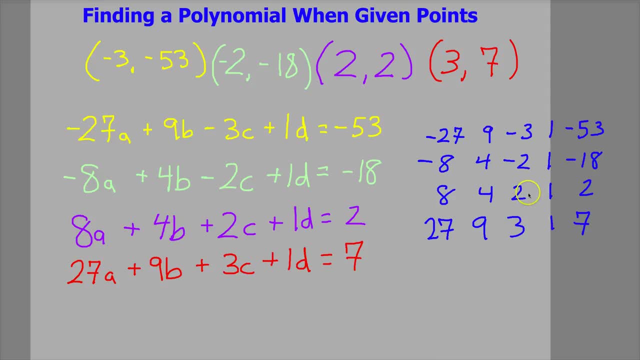 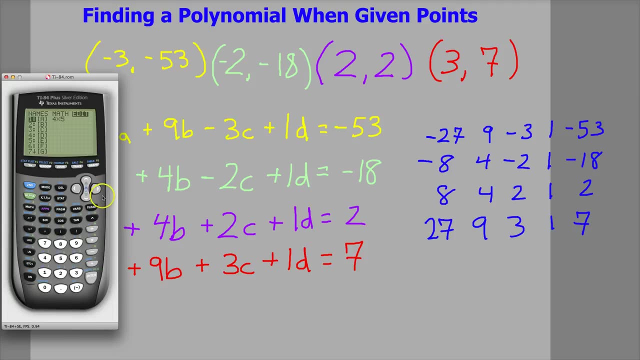 So I have it like this. I'm actually to bring my calculator now. This is the matrix form of what it's going to look like, So I'd go over to wherever your matrix thing is. mine on the TI 84 plus is second and then it's like the fourth button down to see X negative 1 button. so 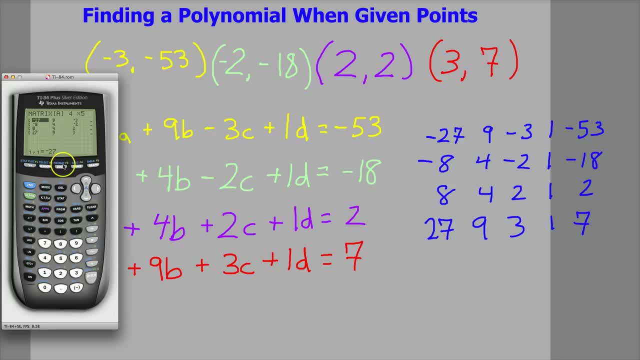 Hit edit and then I'll just go and punch it all in and it should match and you can. once you finish typing it in, you can check your rows. This is a 4 by 5 matrix. in this case, You always name matrices By the number of rows, so negative 2788 and 27 looks good. this column looks exactly like I want it to. this one does as well. 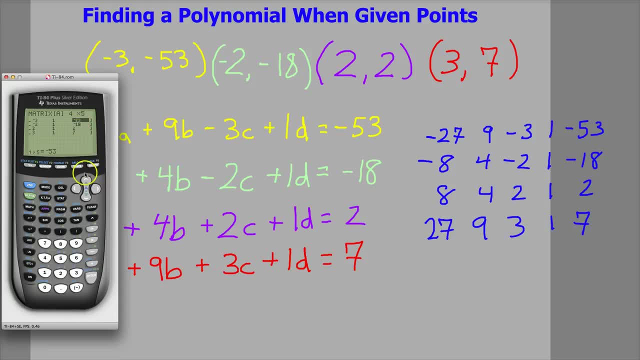 So does this one. And then, finally, This one looks pretty good too. so now that I have that, I can quit out. you do all that work typing it in and I have to quit, but we're going to use it now. so second matrix, and I'm going to go over to the math menu. now I need to go down to reduced row. echelon form. 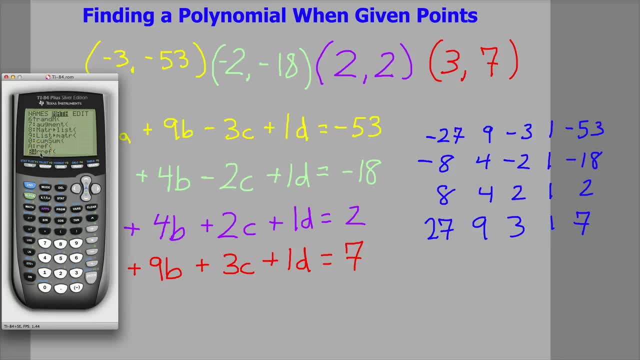 Right here, RREF, don't just do reduced, don't do reduce echelon form. you need to reduce row echelon form. so, RREF, make sure. I think it's B in mine anyway, so I'll hit that, and then I want to hit second matrix again and pick the one I want to apply that to. 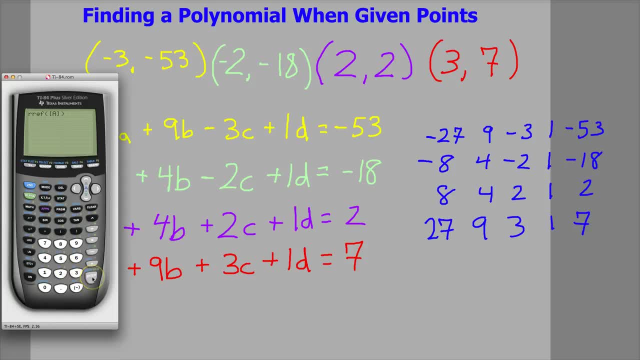 I want to run it with matrix A- whatever you named it- And hit enter and you will get all this stuff. these ones and zeros in the first four columns represent sort of like a light switch. one means it's turned on and zero means it's turned off. so in the first column the only one that's turned on is this top one here, which means that's the value of the term for A. so my A term is going to be one. 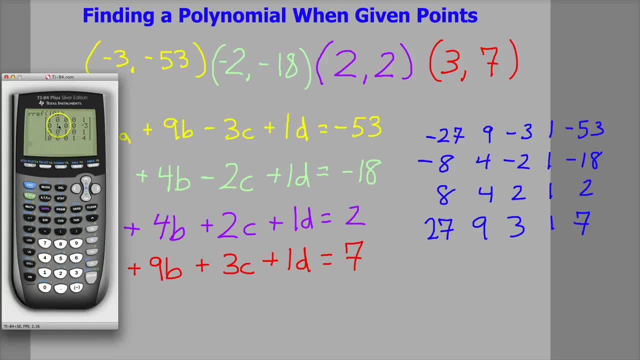 My B term is going to be negative three, because the second row is the only one turned on. third one: This is my C term and finally my D term. so what I'm going to do is turn that into and this will probably drop the calculator up a few times. so my apologies for that. 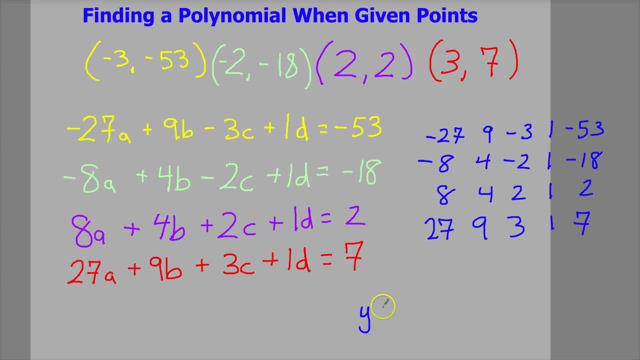 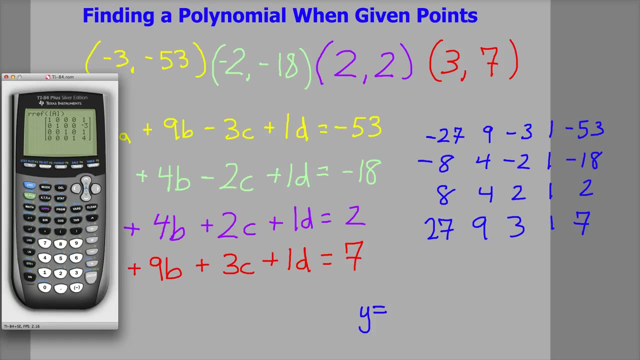 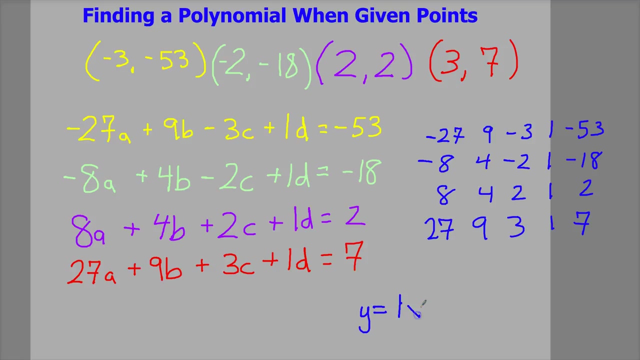 Why so? I use the standard form again. so why is equal to? and in the first case I want to look and see that it's one. so that would be one X to the third power, And for the second set It would be negative three. so minus three X squared. so basically I'm just putting them as coefficients on my variables, and then plus one.